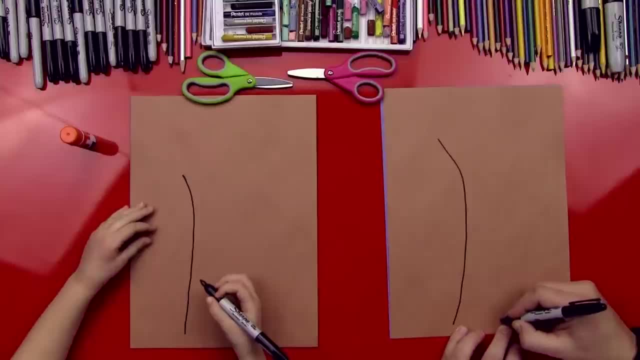 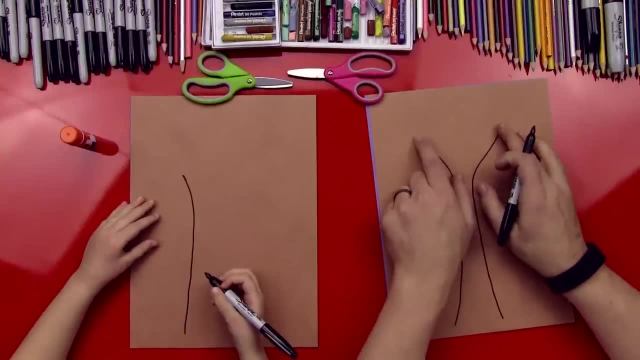 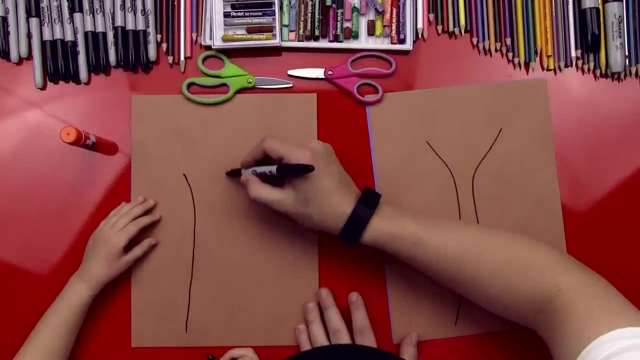 Good, And then we're gonna be over here on this side and we're gonna do another line that comes up and then branches out, And we don't want to branch out too far because then that will go outside of his head. So we're gonna start down here and we'll come up and then we'll branch out off to the side, like that. 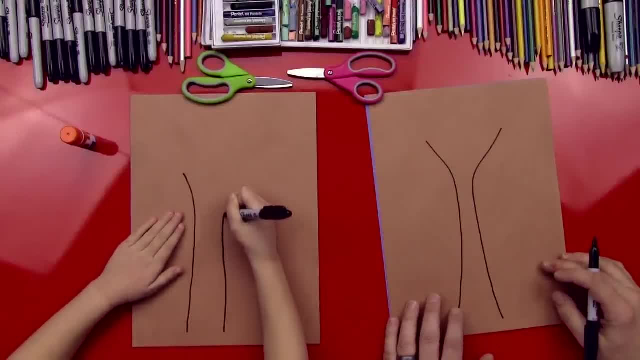 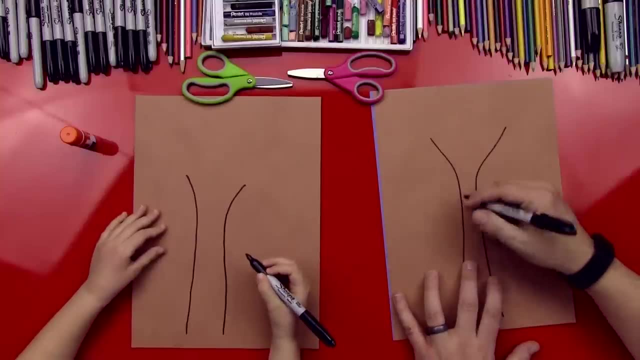 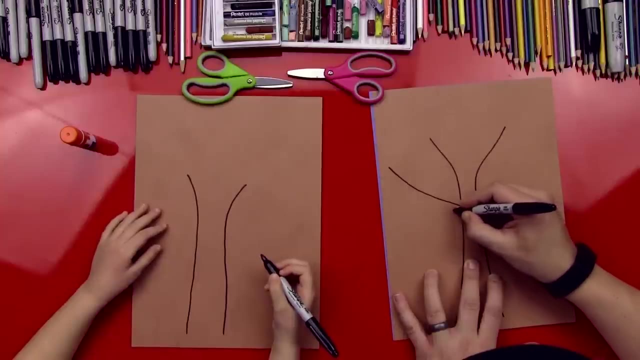 Perfect, Good job. Okay, now we're going to. we're gonna make his arms, And his arms are gonna come out off the side And then we're gonna make. so watch me, we're gonna do a little Y like that, okay. 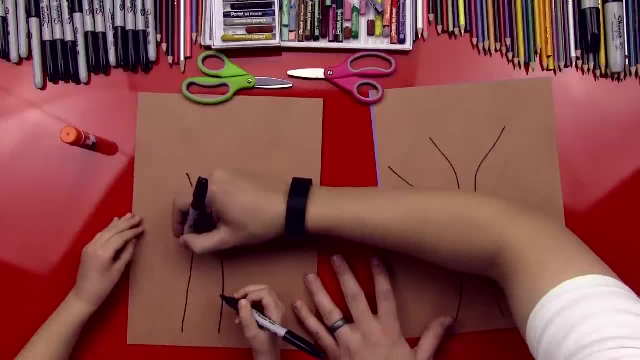 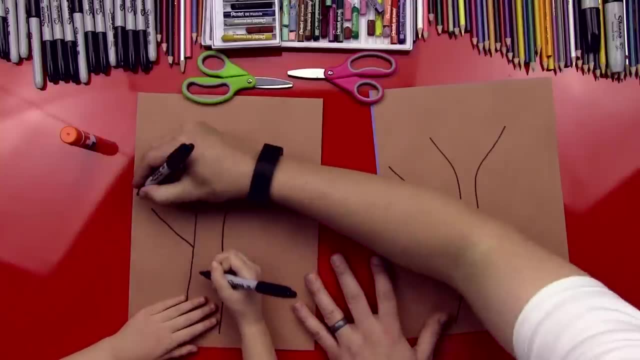 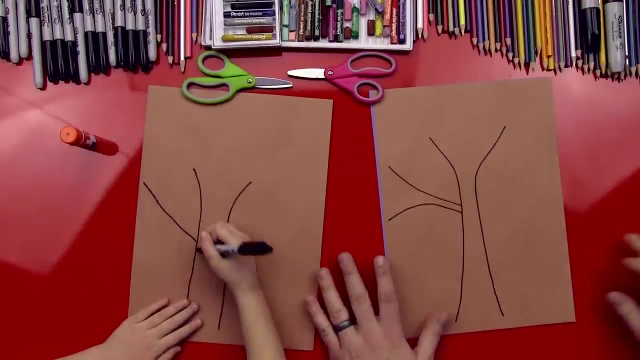 And you do that. So do it right here and go all the way kind of to the edge of the paper. So do one out, Yes, And keep going all the way to the edge- Good, And then come down here and do another one that comes down here. 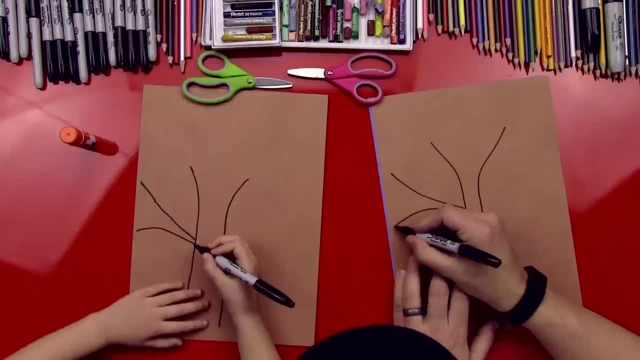 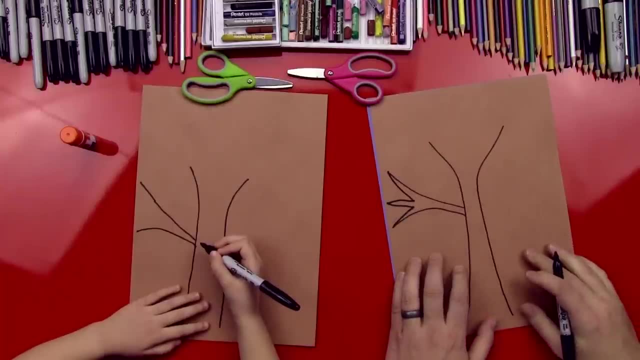 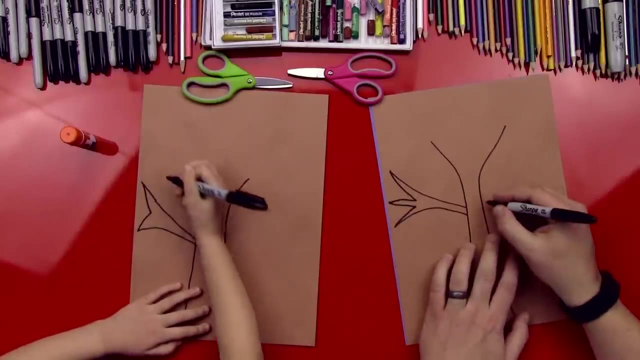 Perfect. Okay, Now we're gonna draw the tree branches inside And this is gonna be for his hand, Okay. So it's kind of a W? huh And that's perfect. Now we're gonna do the exact same thing on this side. 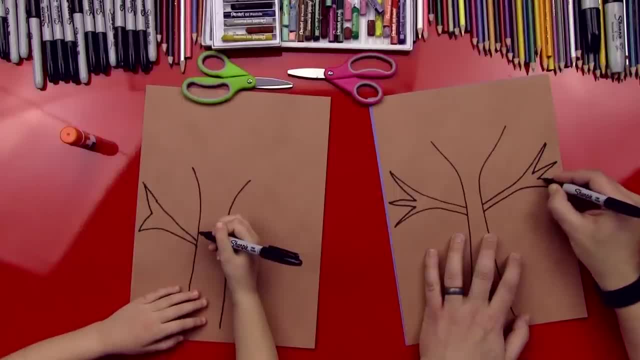 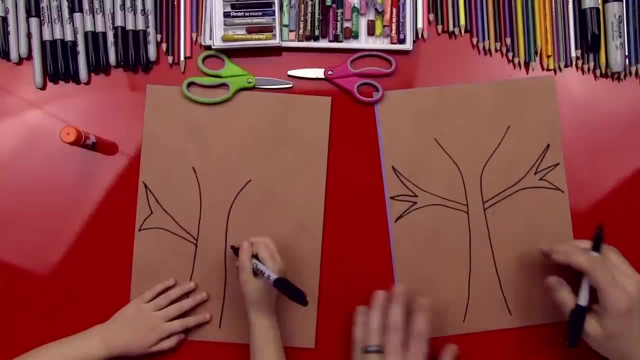 We're gonna do this is gonna turn into his hands. It might be kind of confusing what we're doing, but you'll see what's gonna happen. It's gonna be really neat. So we're gonna do the same thing over here. 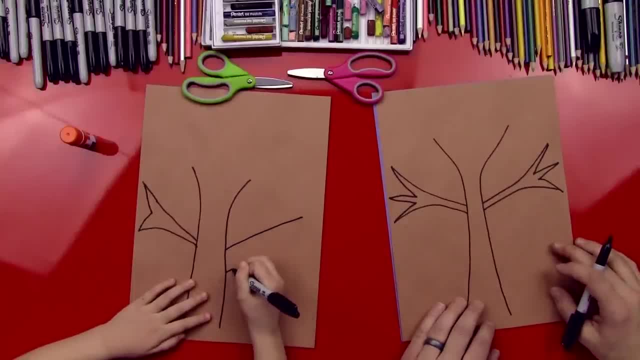 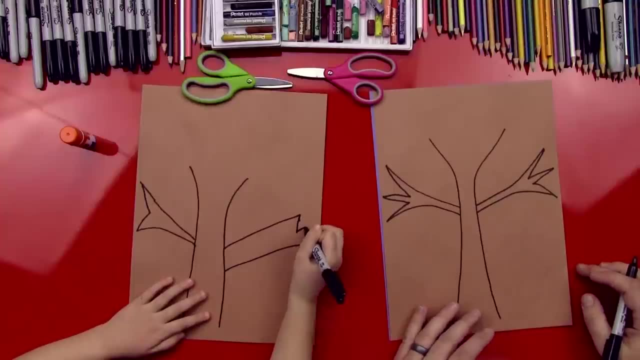 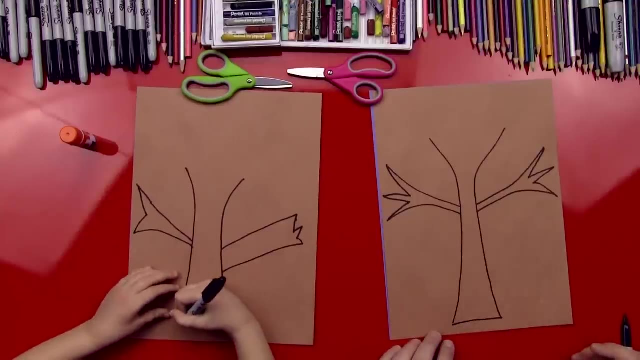 Draw another branch that comes out over here- Good, Well, that's gonna be a big one- And then do a W in there for his, or a V, Yes, Okay, And then we can just draw a line that connects the bottom. 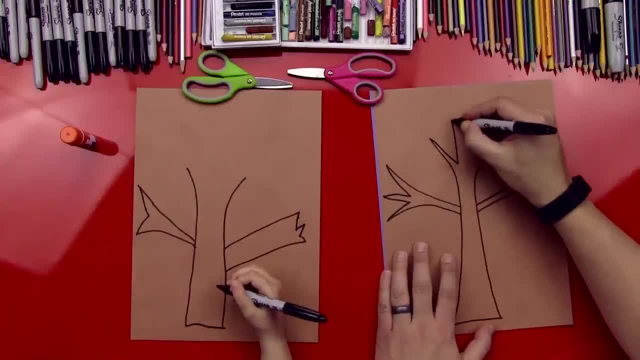 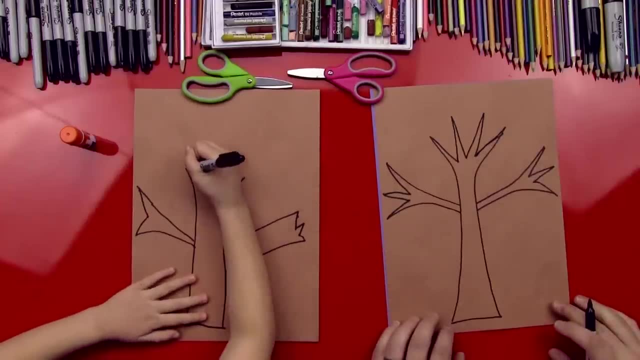 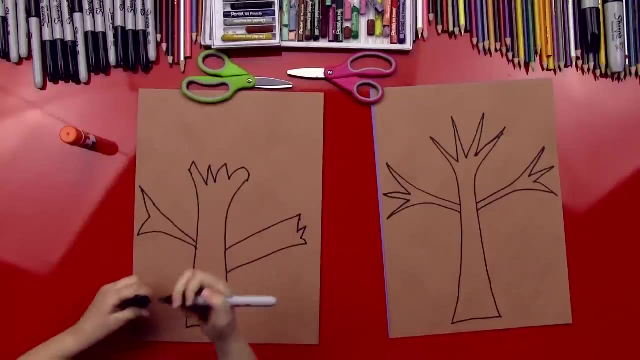 And then let's do a W up here for the branches up here. We can do a couple, I'm gonna do a couple. Oops, There we go. Good job, Perfect. Okay, Now let's cut this out. We're gonna fast forward, all right. 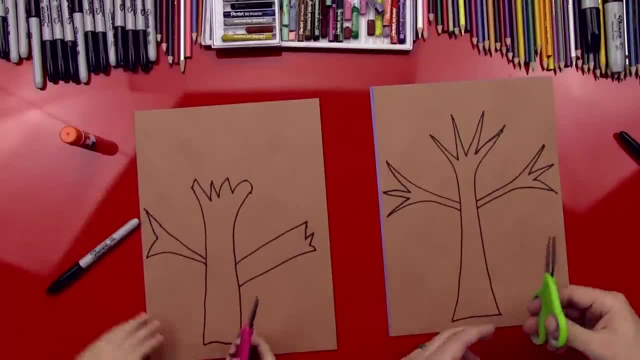 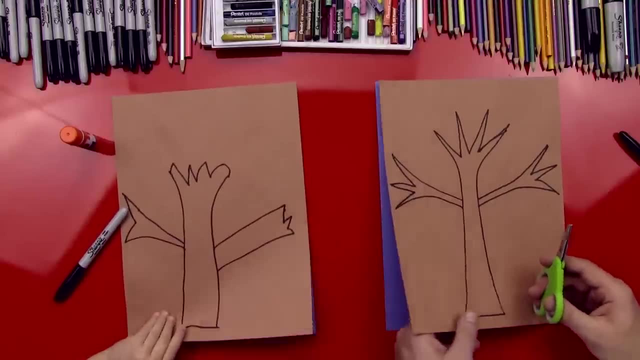 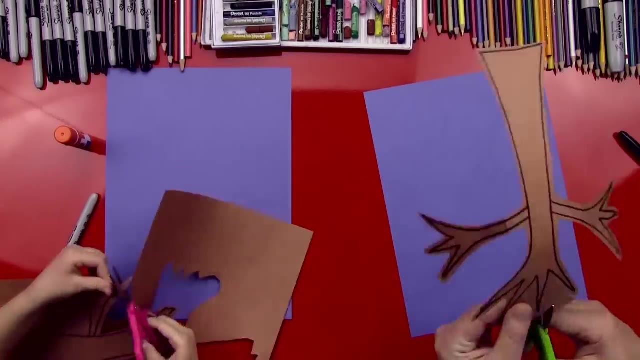 And our ERP friends. you guys can pause the video and then cut yours out if you're following along with us, And then, once you're done cutting it out, you can start the video back up. All right, Yeah, All right, Right now. 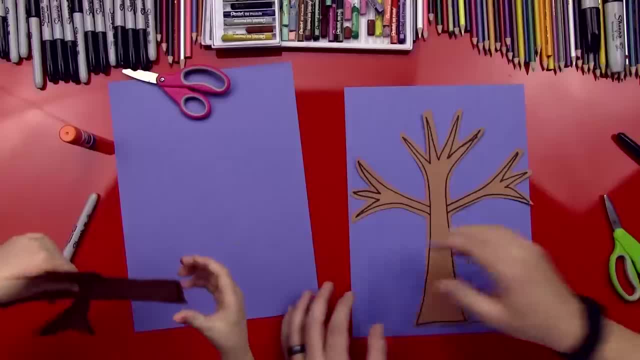 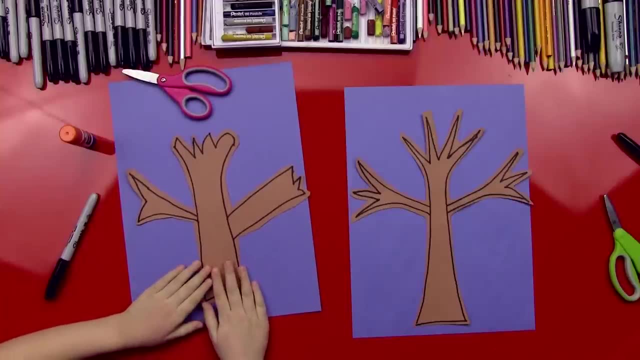 Good job, heads. You got it all cut out. Let's see how cool he looks. Oh, that's awesome. That's gonna be his bones. Okay, Now we're gonna get our white piece of paper And we're gonna need two sheets. 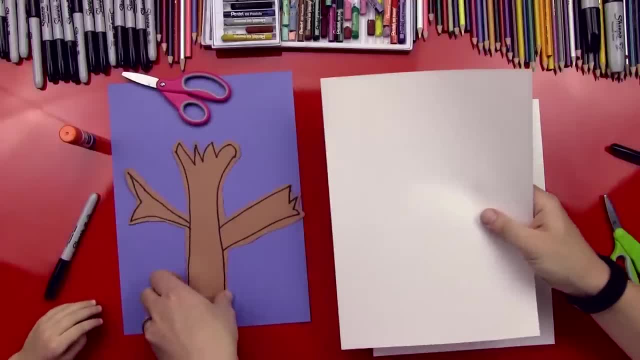 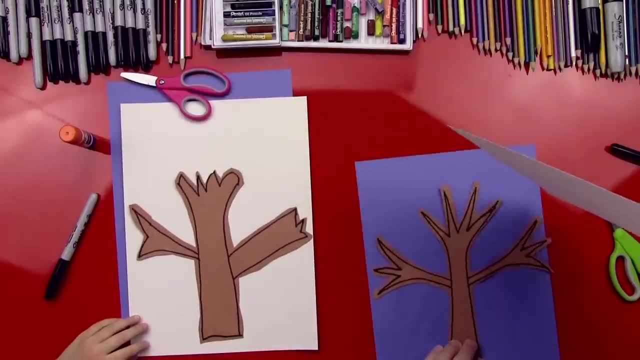 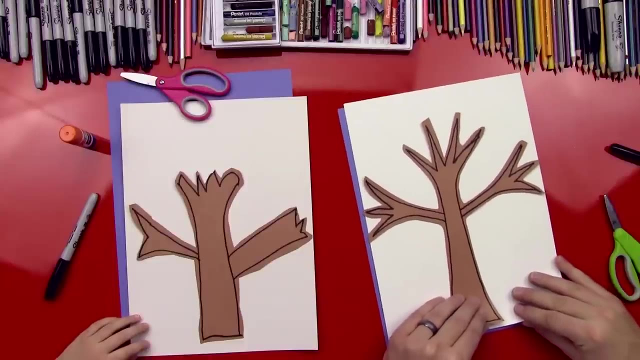 For each of us. Okay, So we're gonna put this under the tree first, because we're gonna trace our snowman next. Okay, So we're gonna do this. We'll put this like this And I'll show you why. we'll need two pieces of paper. 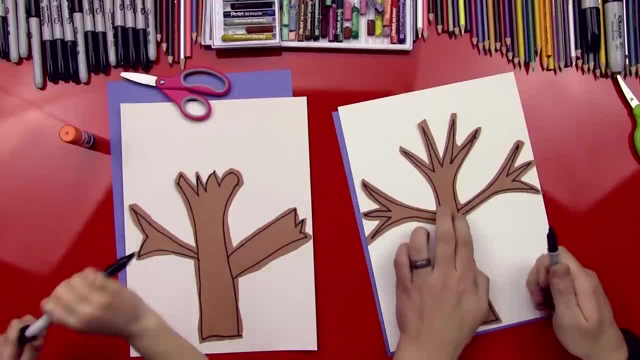 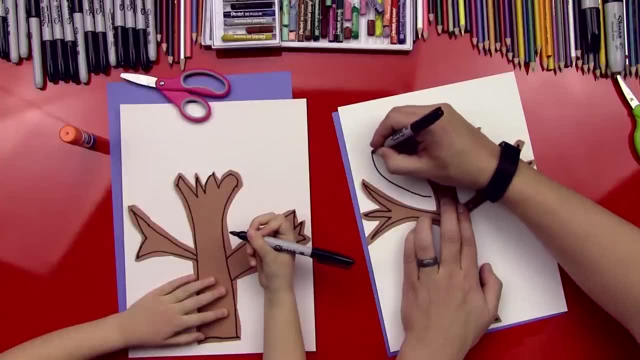 But we'll just start with this first. Okay, So get your marker, And then we're gonna draw his head first. So we're gonna draw a big oval. That goes: You're wobbly. Yes, I'm really wobbly. 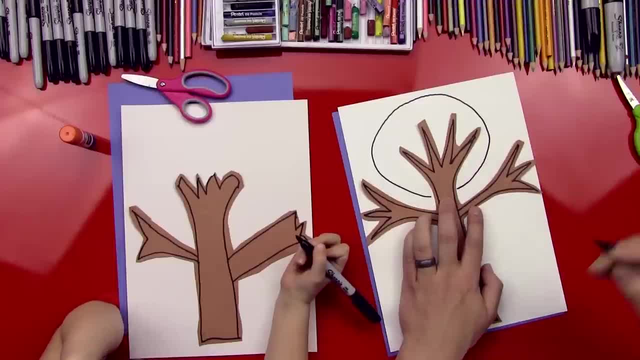 Thanks for pointing that out. So there's the snowman's head. I'll straighten it just for you. Okay, So you do your snowman's head. So you start here and go around like that And you don't wanna draw on your tree. 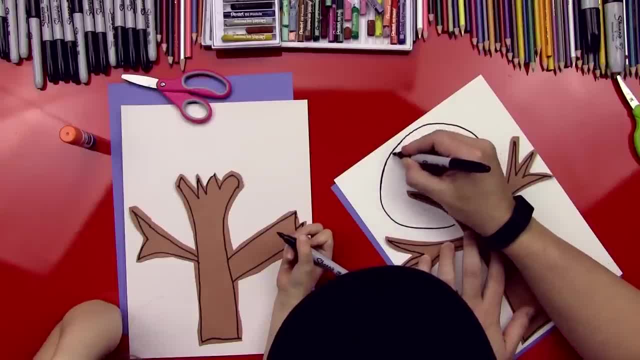 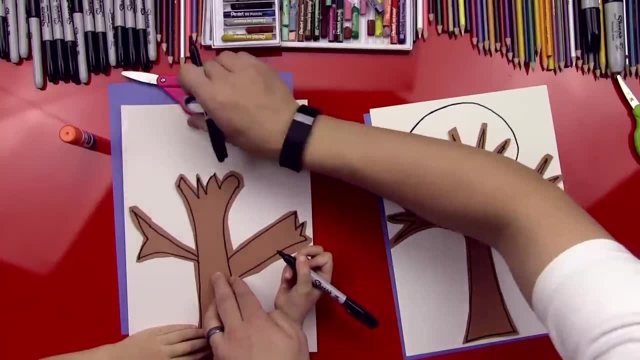 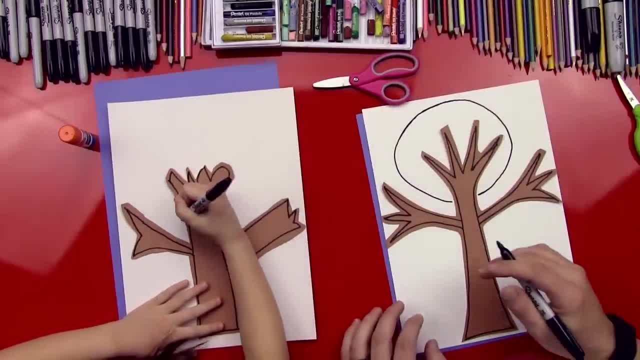 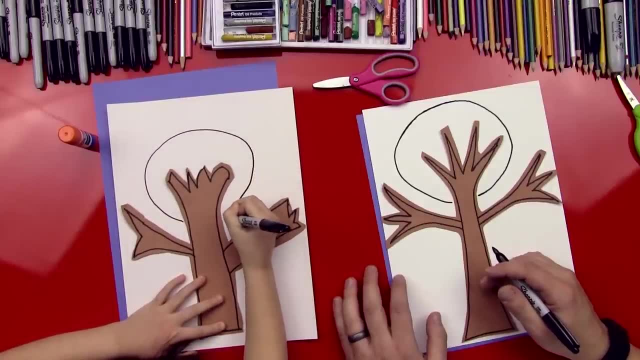 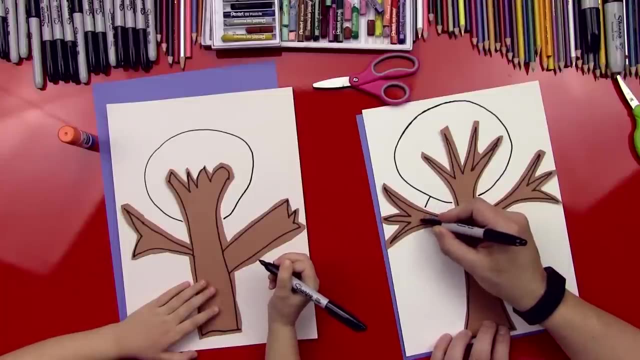 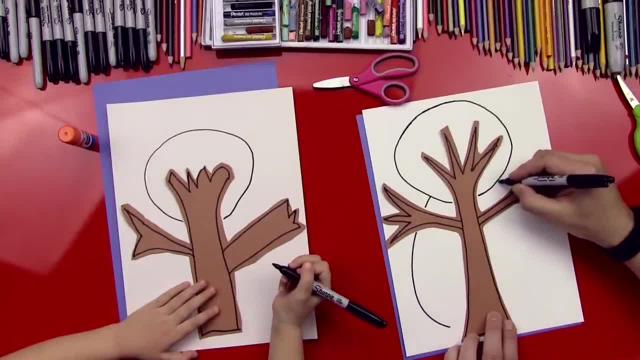 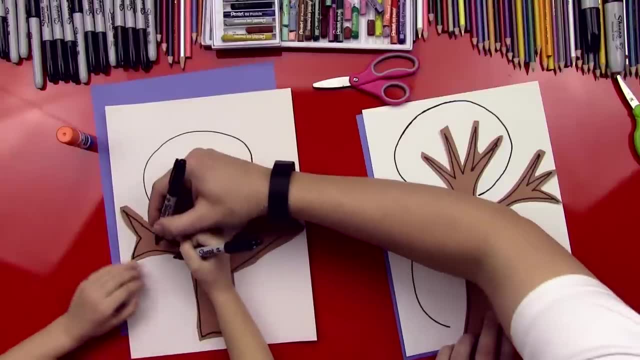 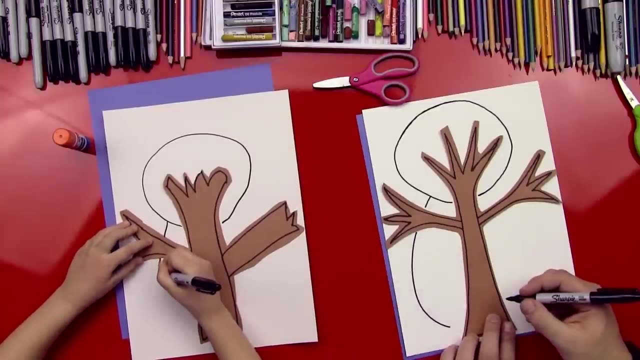 And we're gonna do the same on this side. So you go ahead and do that. You do start right there, Draw a little line right there, Good, And then draw another line- Let's start right there there- and does kind of makes a J backwards, J yes, and then in, and then. 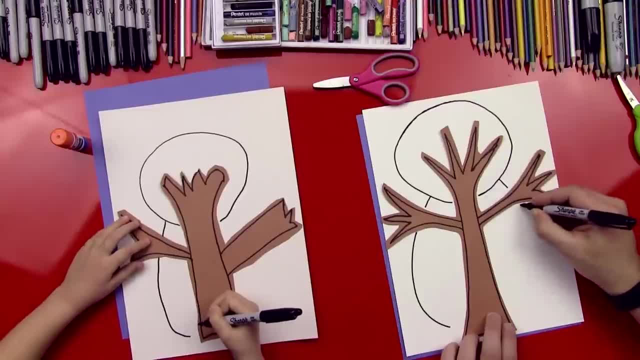 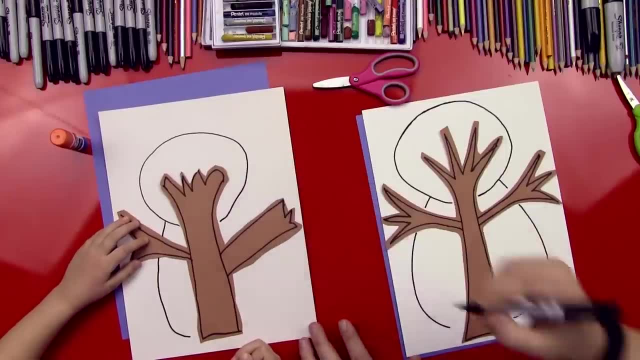 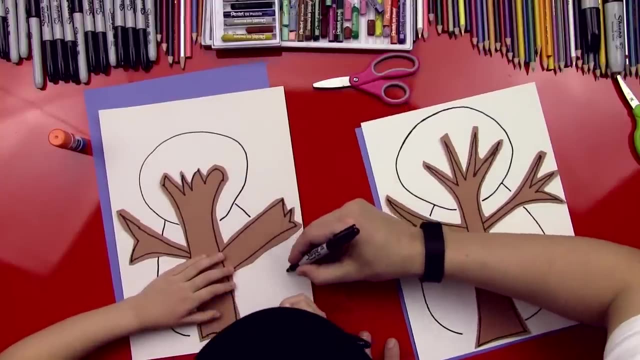 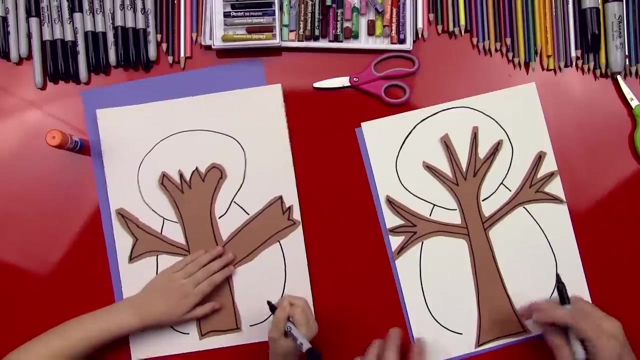 we're gonna do the same on this side. come over here like that, this side draw a little line right there, right there, good, and then imagine the line right here coming over and good, okay, now let's move our tree out of the way, and then we're gonna connect these lines. 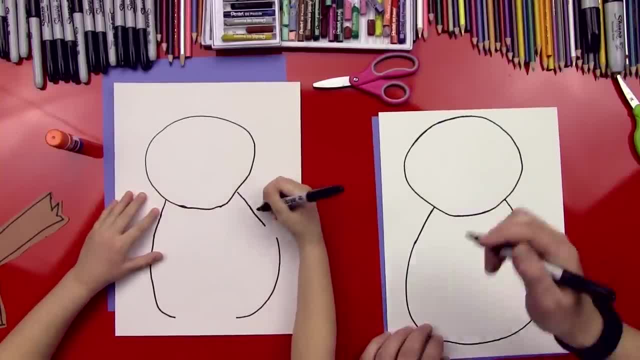 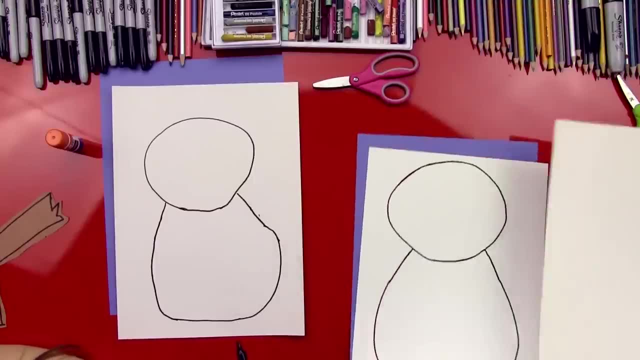 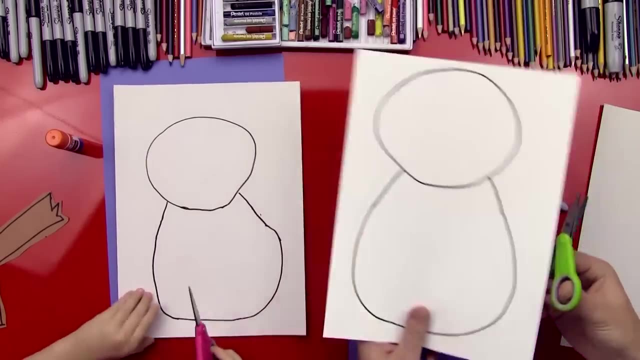 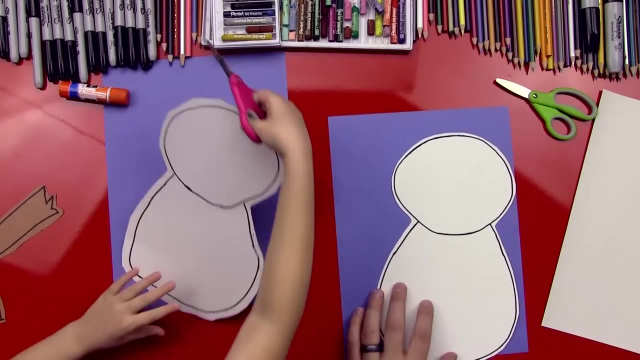 but my snowman looks funny. good, and then connect the bottom. now we are ready. let's cut this out first, and then we'll use this, this next sheet of paper, after that. so let's speed it up ready. perfect, you got it. good job. okay, now we're going to glue our tree down first. 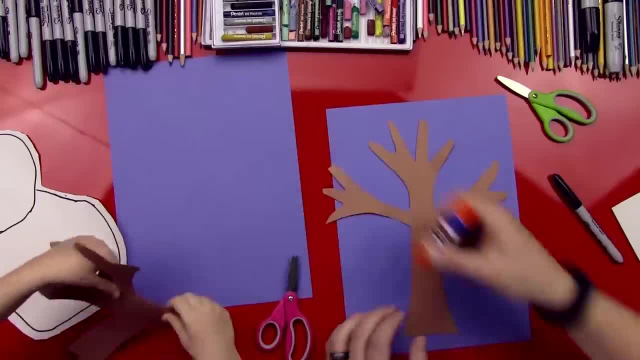 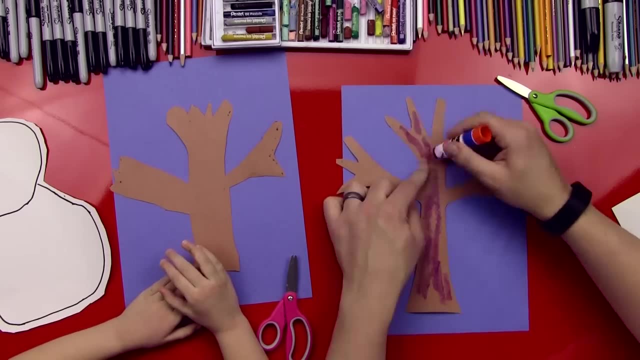 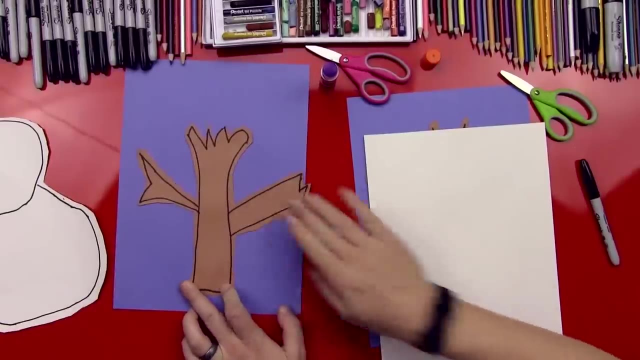 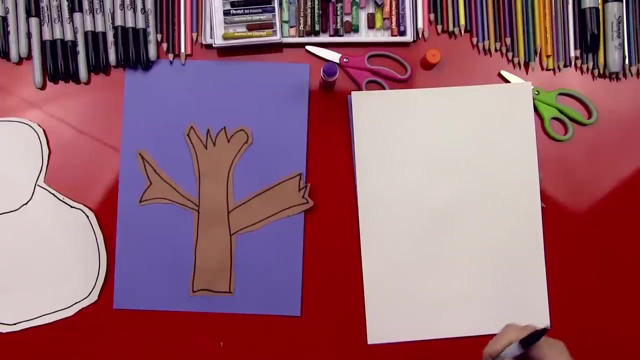 or next. so we get turn them over and we're gonna get our glue stick and make sure we get him covered in glue. good, you've got your tree stuck down. now we're going to drop. now we're going to draw the snow at the bottom of the ground, on the ground snow, that's on the 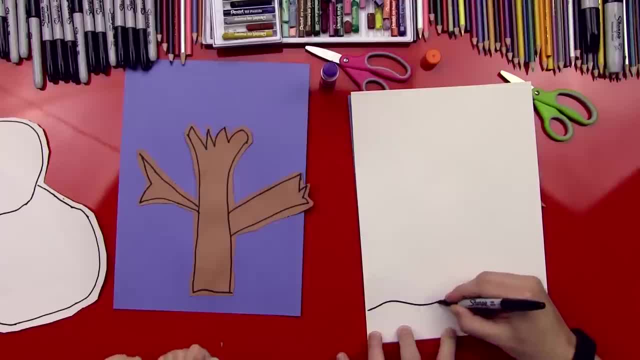 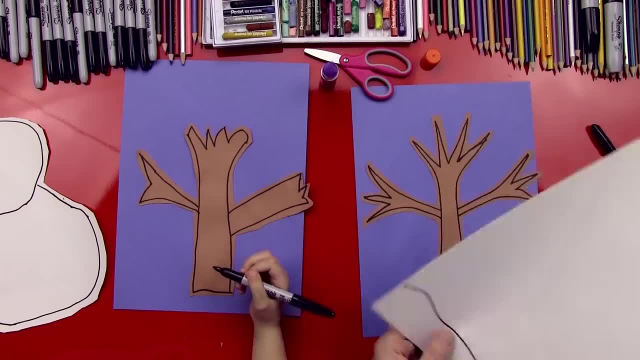 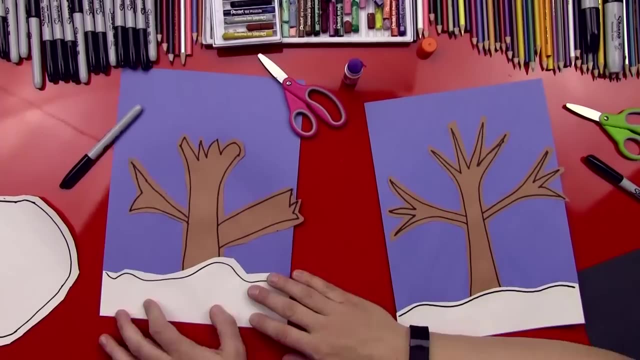 ground. so we're going to do: I'll give you this paper in, just so I'm going to make kind of a wavy line, it goes like that- and then I'm going to cut it out and we'll glue this down. Okay, we got our snow all glued down, right, Yeah, Yes, Okay, now we're going to move this. 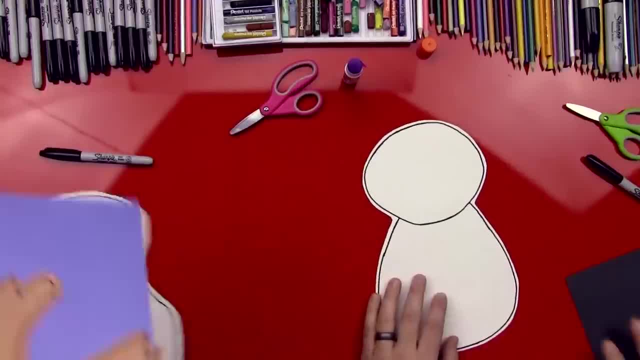 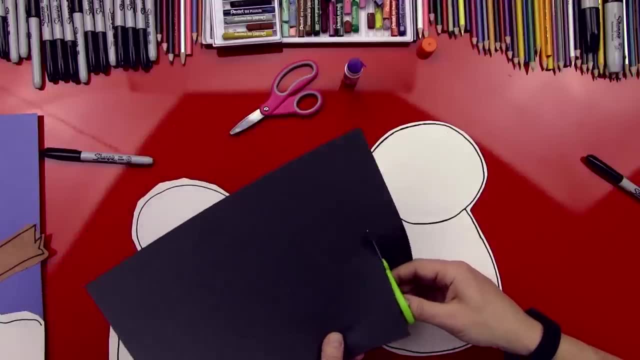 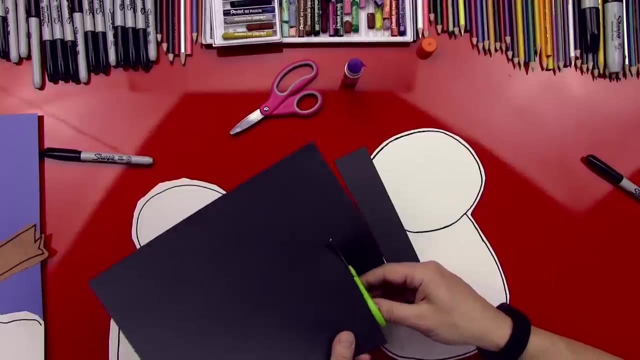 off to the side and we just want our snowman. Okay, we are going to cut a little strip of black off the edge of this paper, this sheet, and I'll show. we're going to do a little trick. This is going to be really cool. Do you know how to make a fan? No, You don't know how to make a fan- No, 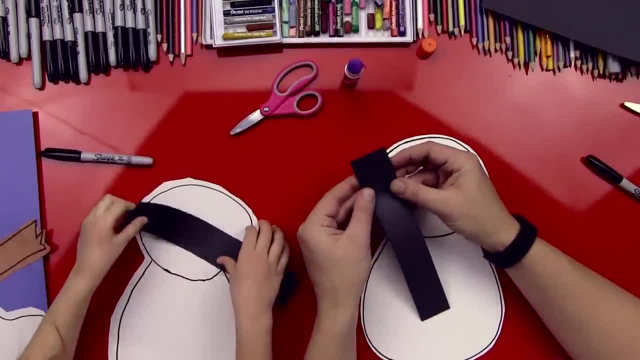 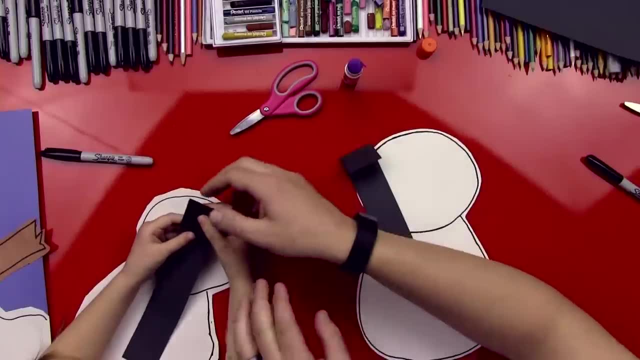 But you did. All right, we're going to do, we're going to take our strip, we're going to fold so that this first fold makes a square. You see that? So fold it down. There you go, That's perfect. 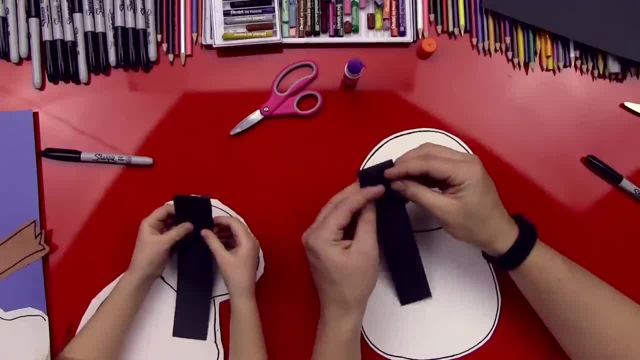 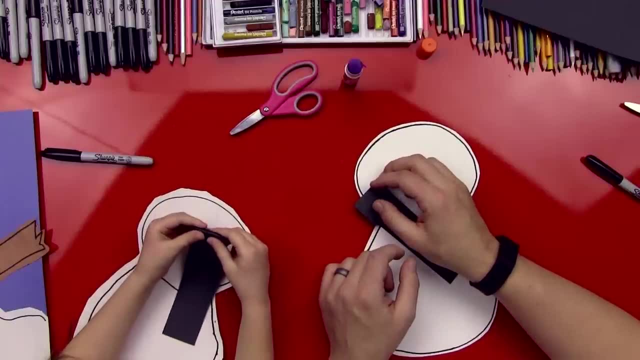 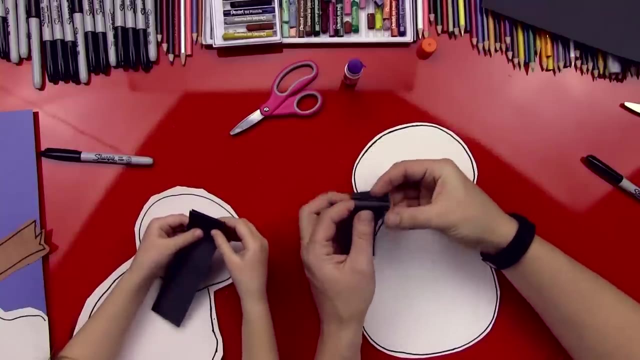 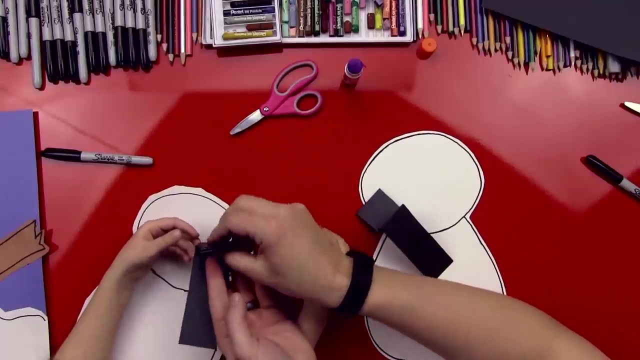 And then fold it. Good, Okay, now we're going to fold it back this way, Yes, Perfect. And then squish it. Okay, and then we're going to fold it back the other way. Did you do it? Let me see? Did you fold? Oh, yeah, you're right, You did it. Okay, squish that. 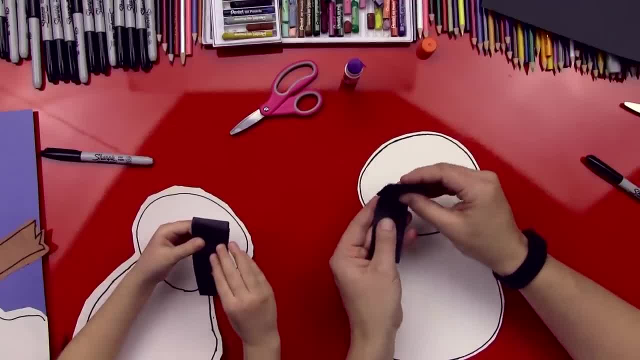 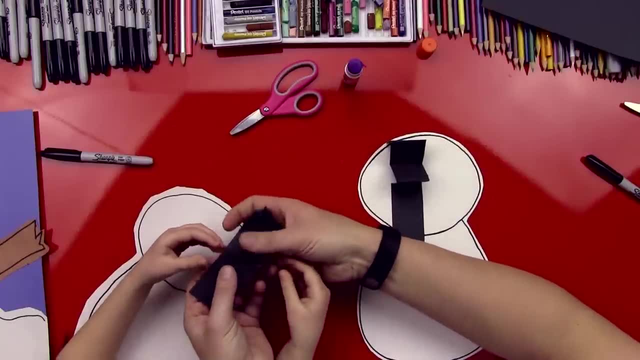 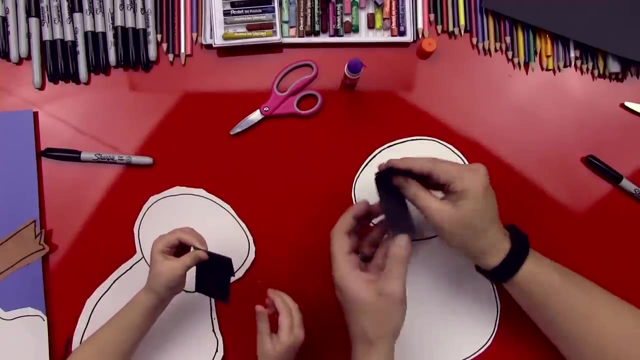 Good, Okay, and then we're going to do one more back the other direction. Let's see, You want to save the paper, I'll help you. So you do that right on the edge, like that. Good, And then one last one. There we go, Now fold that last piece in. 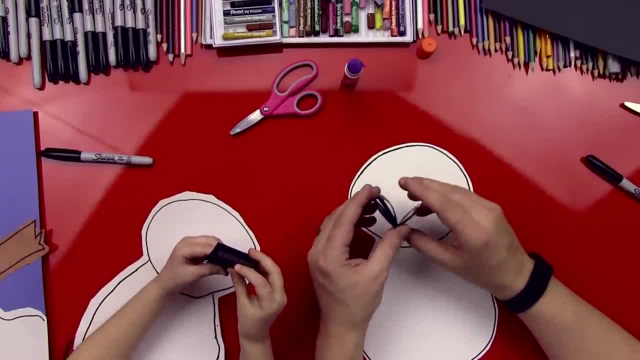 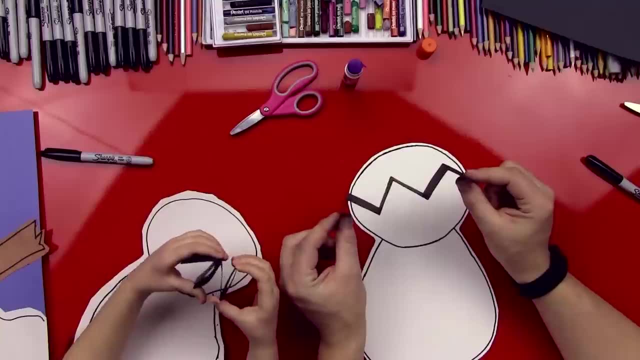 This one. Yes, So it should look like that, Like a zigzag. Is that cool? Yes, Okay, and then we'll squish it back together And we're going to take our scissors and we're going to make a circle. We're going to cut a circle. 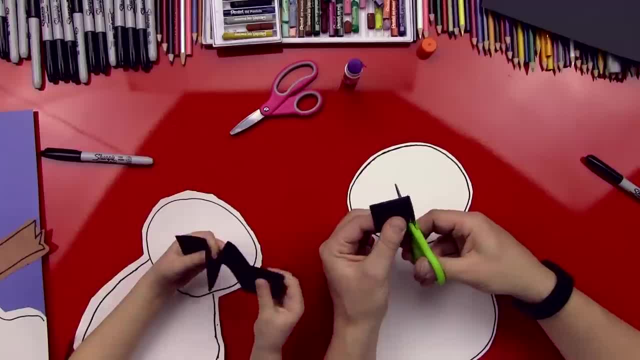 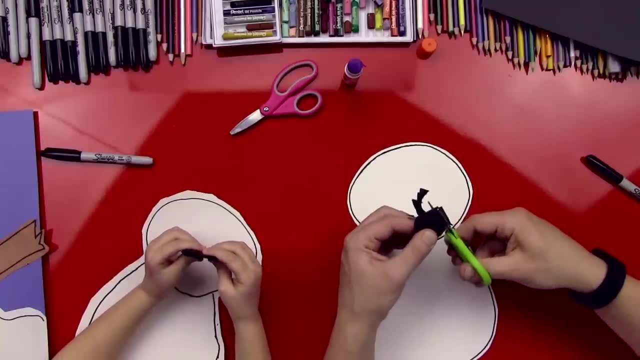 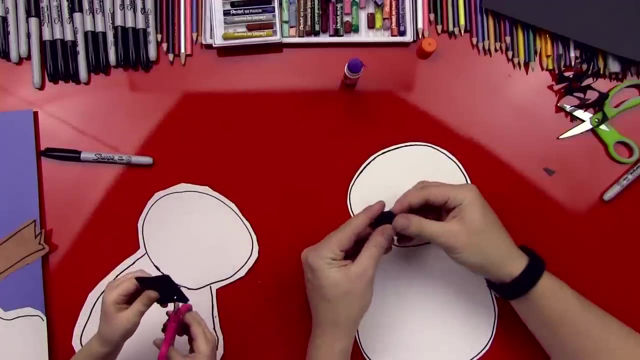 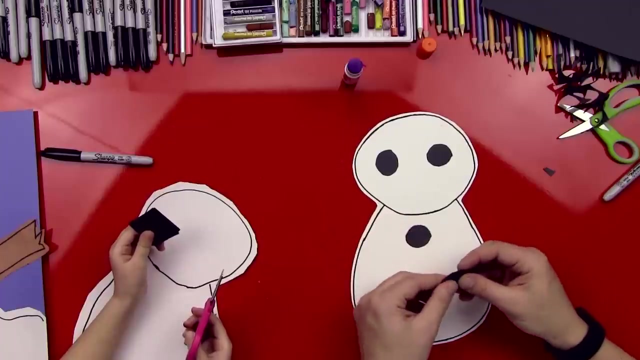 out of our fan or a zigzag. We cut a big circle all the way to the edges, like that. And then, when we're done, look at this, We've got an eye And we've got buttons for his belly. Is that cool? Yes, So go ahead and make a circle. 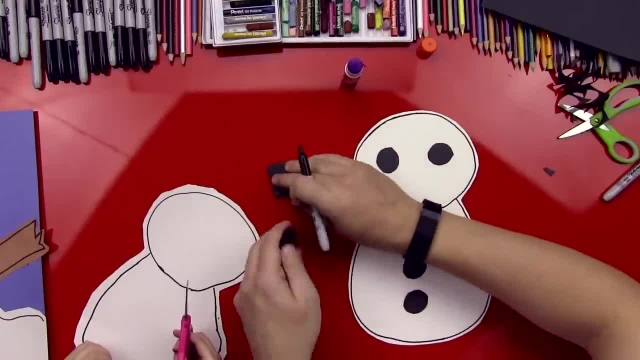 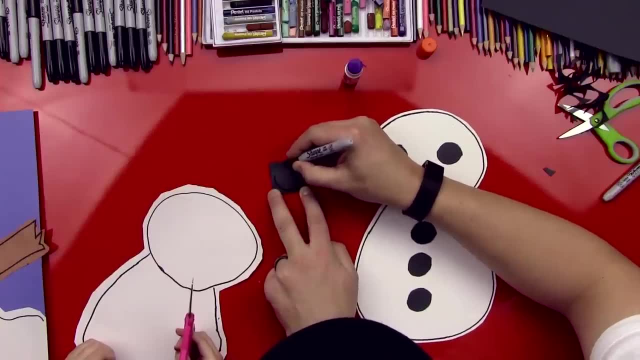 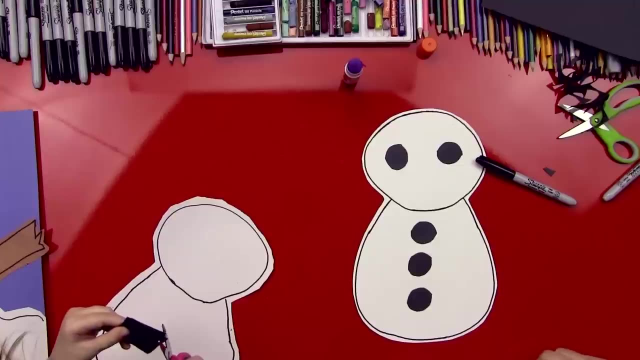 Let me, I'll draw it. You know what, If you're doing this with your parents and you're kind of young, you could actually ask your parents to draw a little circle on the zigzag and it might be easier to cut it out. Whoa boing. All right, let's speed it up right now. 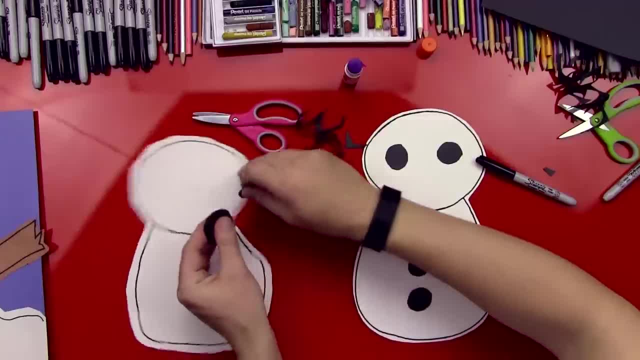 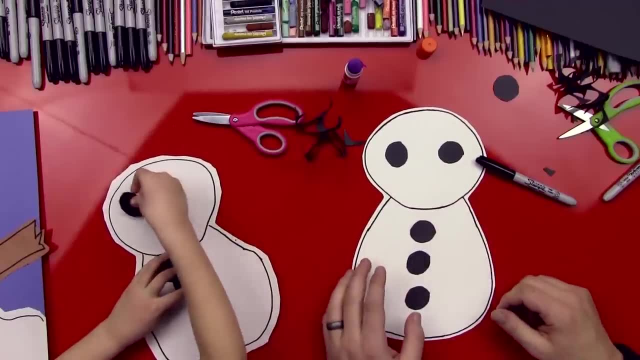 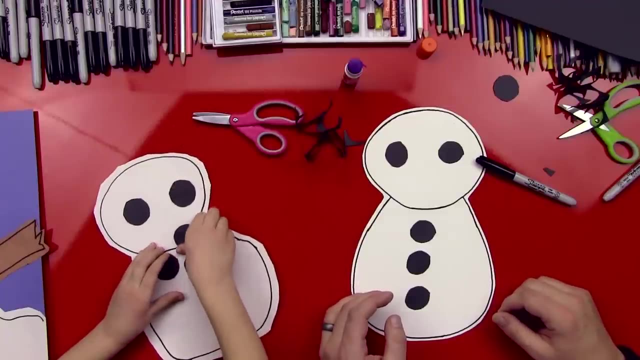 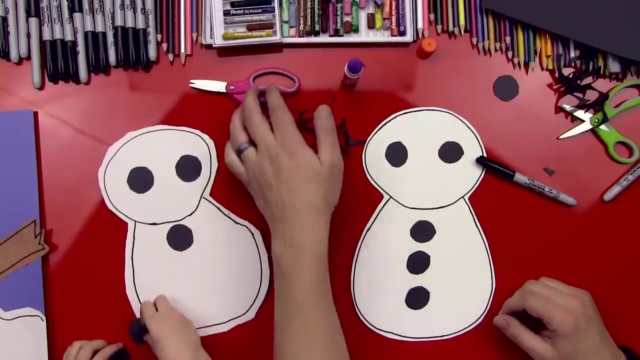 So that was a little hard for you. huh, Yeah, You asked me for help. Yeah, All right, you want to put your little eyes on there and the buttons One, two and then put three buttons: One, two, three. Okay, 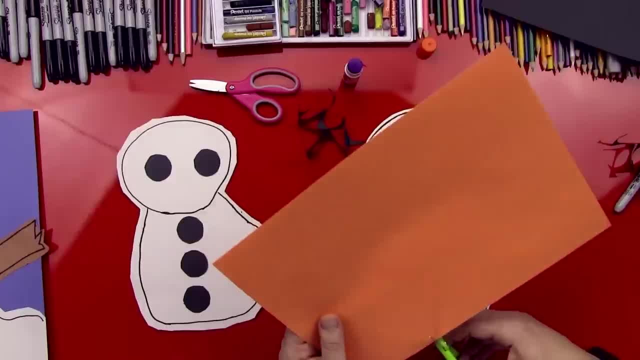 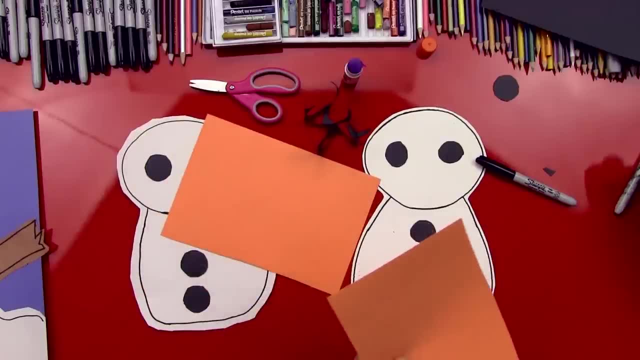 Now we're going to do a carrot for his nose and we'll just use half a sheet. We don't even need half a sheet, We'll save. We'll save this because we're not going to use all of it. We'll put this: 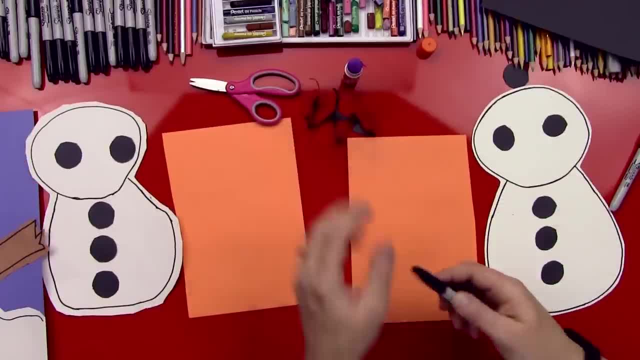 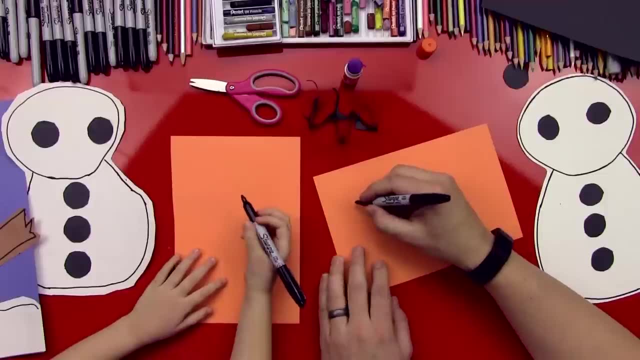 off to the side and we're going to draw a carrot. now I'll show you how to draw a carrot. You got your marker, Okay, We are going to make a wiggly V, All right. Well, let's do a C first. We're going. 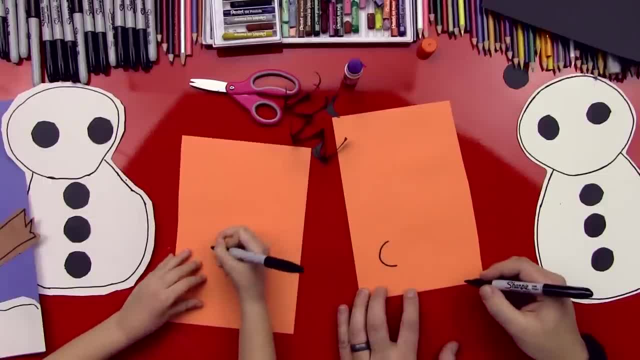 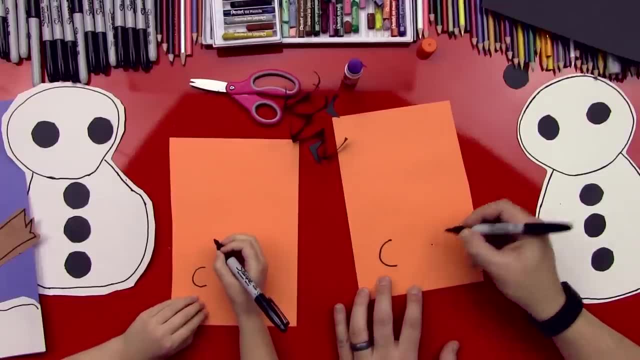 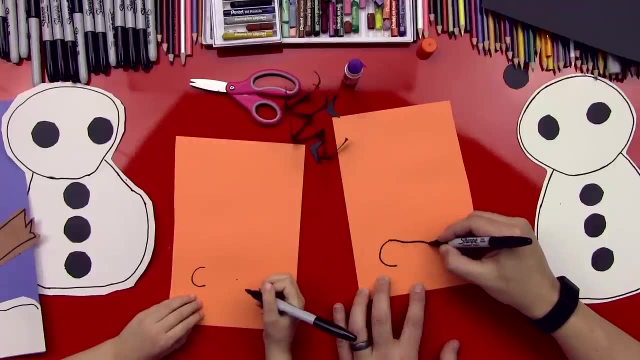 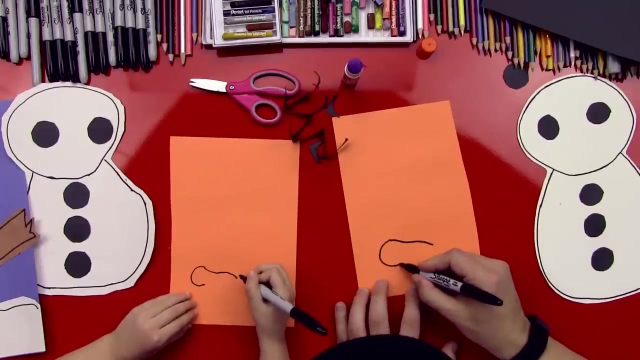 to do a C, Okay, Good. And then from the C, let's put a little point out here: Boink, Okay. And then we'll do a little wiggly line to the point: Good job. And then we'll do another wiggly line to the point. 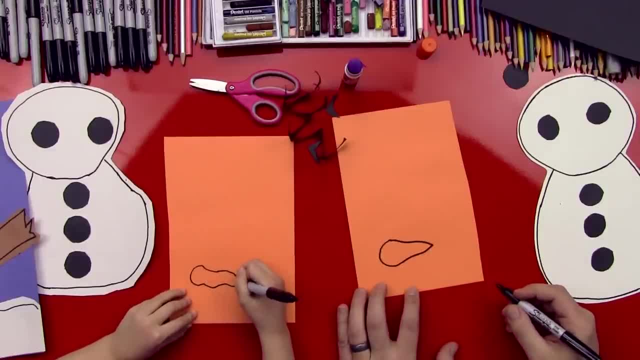 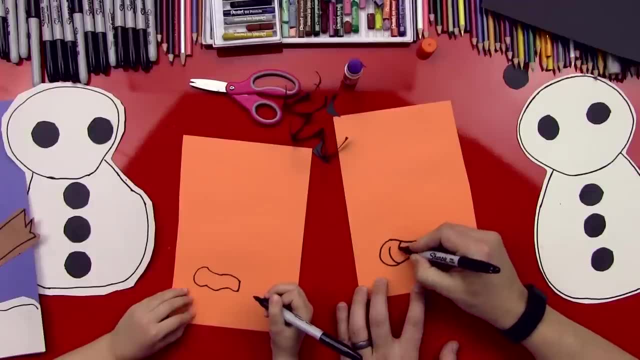 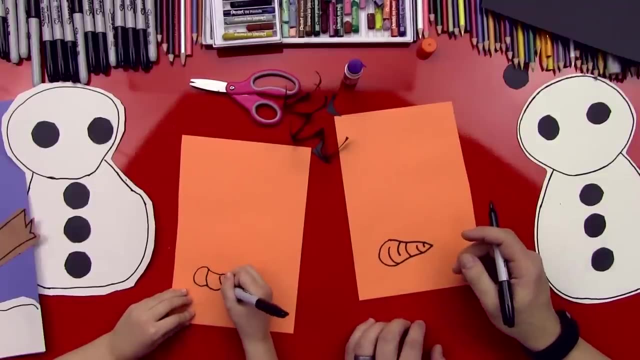 Right to the point. Oh good, I like it. Okay, Now let's do some more Cs, And this is going to be for the wrinkles on the carrot. Do that? Good job, Perfect. Okay, Now let's cut out our carrot. 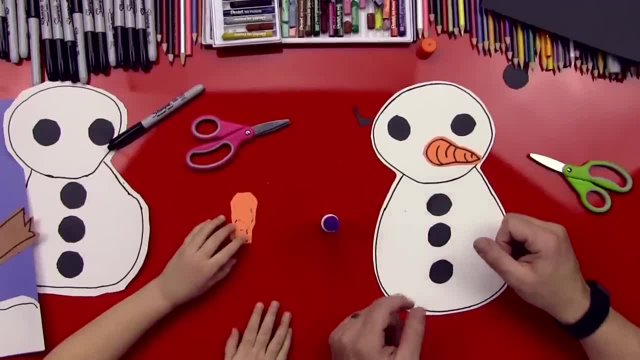 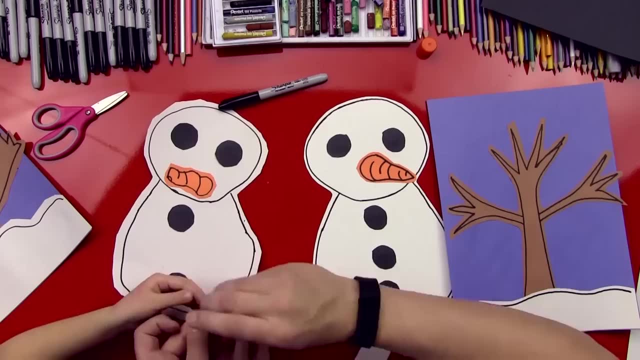 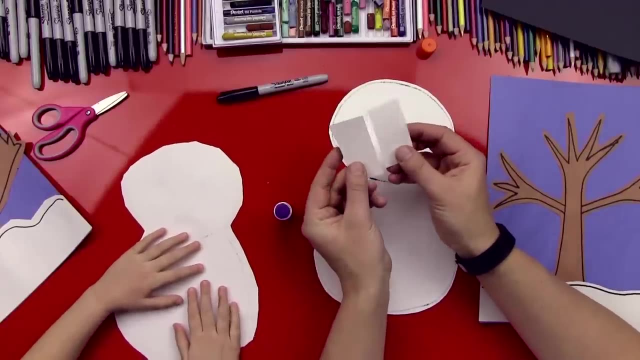 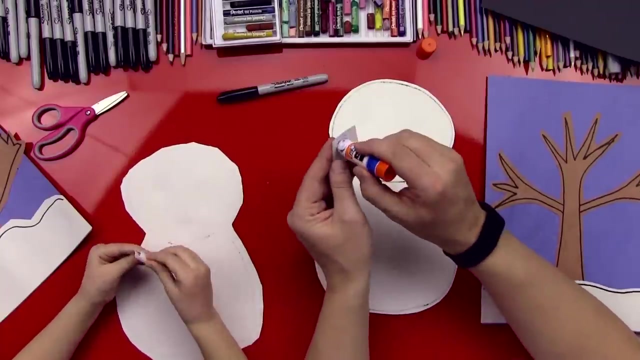 Okay, So we got all our pieces cut out. Let's glue them all down now. Next step: we're going to flip our snowman over and I cut out these little rectangles. You'll fold your rectangle in half. Good, Then we're going to glue one side like this and we're going 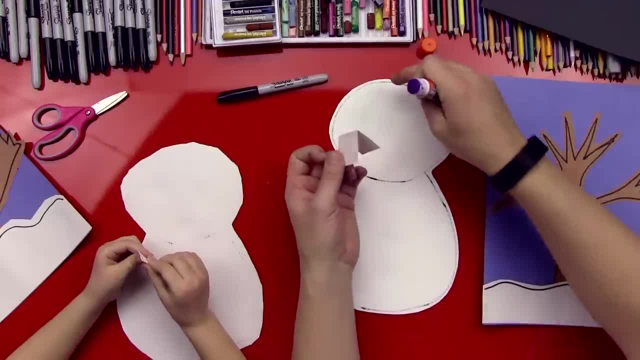 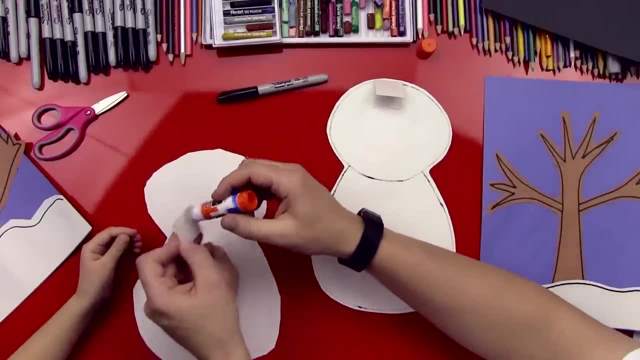 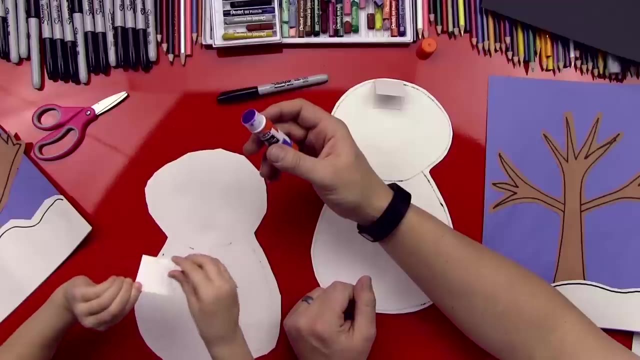 to put the folded side, this side, up at the top of his head, just like that. Can you do that? So let's glue this, Okay, Good, and then what side goes up at the top? the folded? yes, there you go and put line it right up at the. 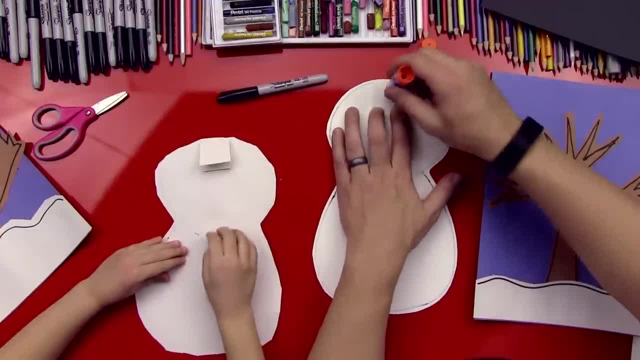 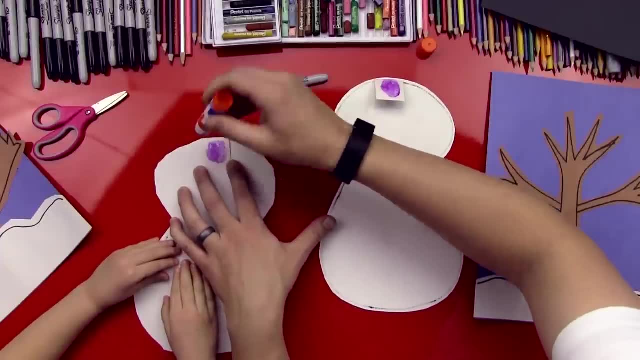 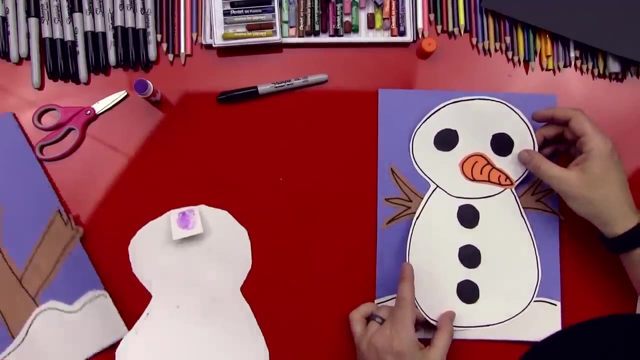 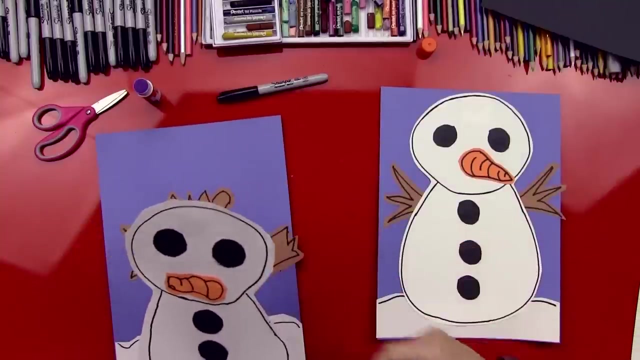 top. perfect. now we're going to glue this side and this is where it's going to be really cool. snowman told you it wasn't going to be boring, huh? we're going to flip him over and we're going to line him up with our tree and then stick it down like that. so go ahead, you line it up and then stick it. 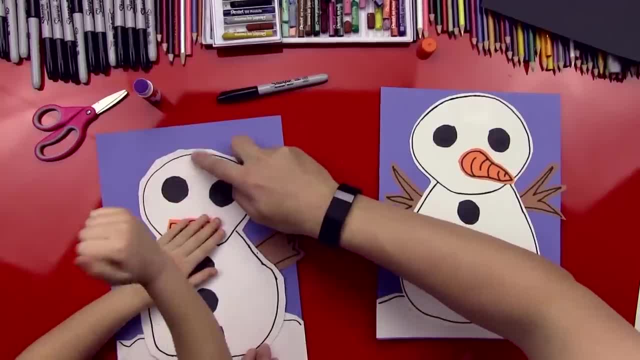 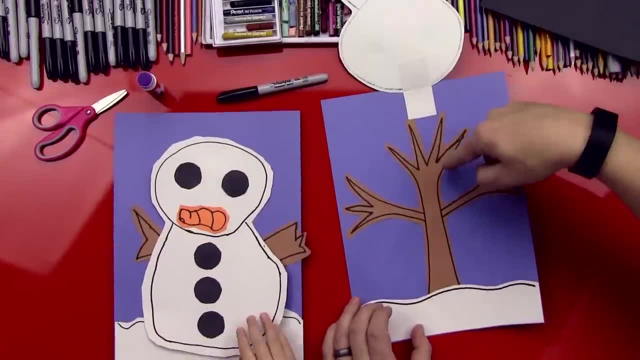 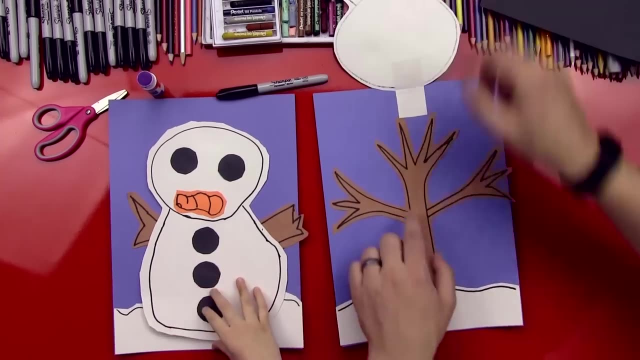 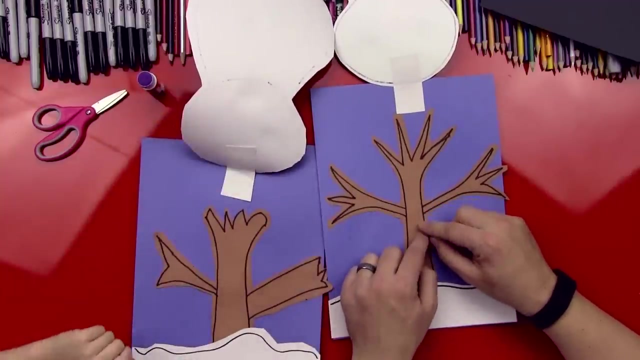 down, squish it right there, smack it. good job, now watch this. we can open them up and we can see the tree underneath. huh, is that cool? yeah, that's pretty neat. so what we should do next is we should do something really cool on the tree. we could draw birds. we could cut out a heart. we could put a heart right here. 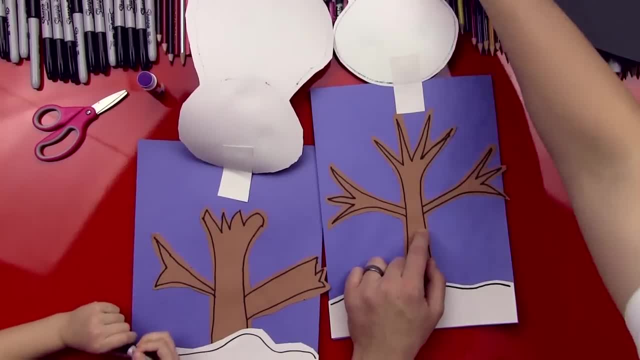 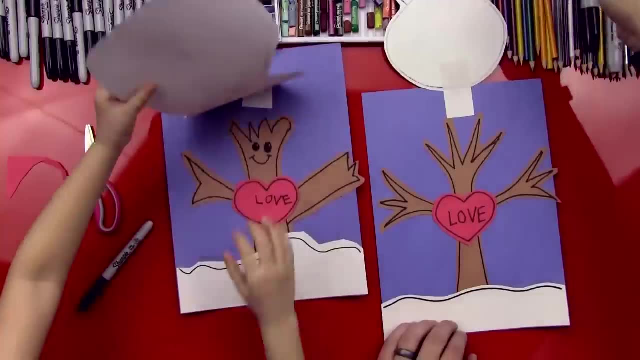 we could do a little face on our tree. should we do that really quick? yeah, all right, okay, heads. did we put something special in our snowman? yeah, what did we put little hearts? ah, it's so cute and you did a little face. it kind of looks like Groot from guardians of the galaxy. 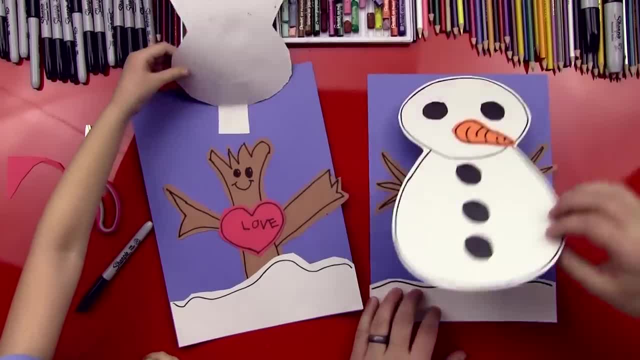 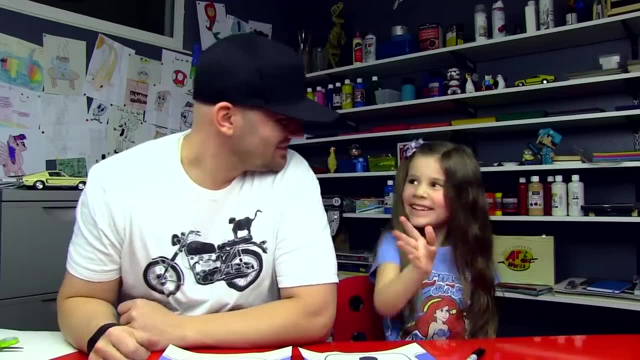 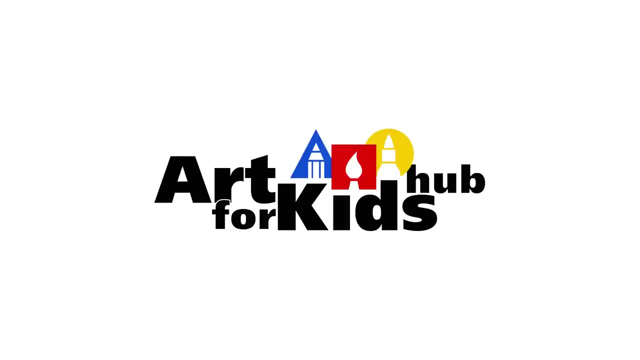 he looks awesome. did you have fun you promised? we hope you guys had a lot of fun making your snowman's with us and we'll see you later, our friends, goodbye.